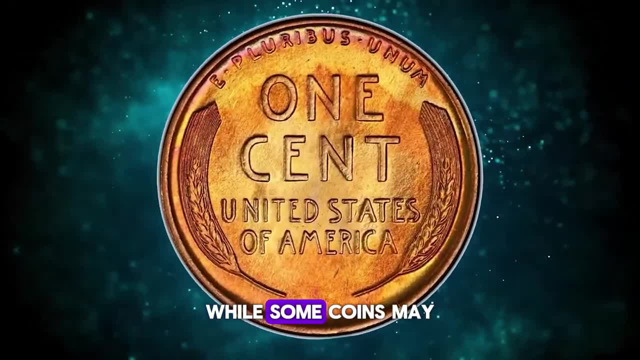 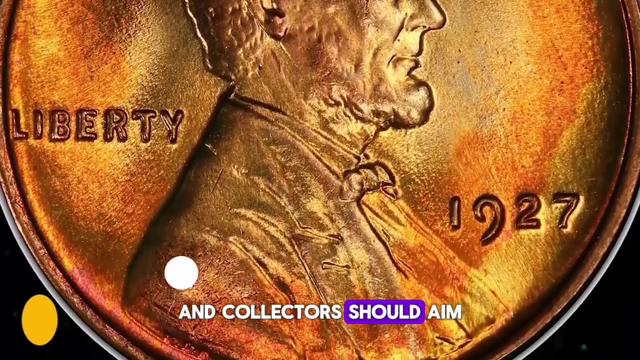 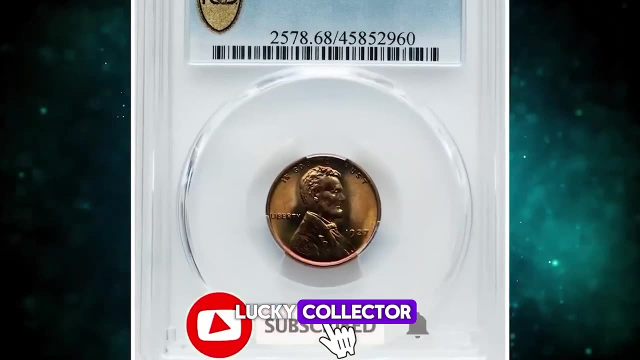 above the grade of MS66RD. While some coins may exhibit less than full strikes, this is not a major concern with the 1927 P cent, And collectors should aim for nothing less than a sharp impression. This elusive specimen found its way into the hands of a lucky collector, fetching an impressive 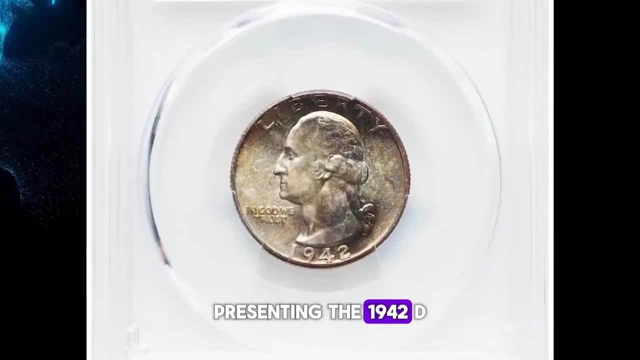 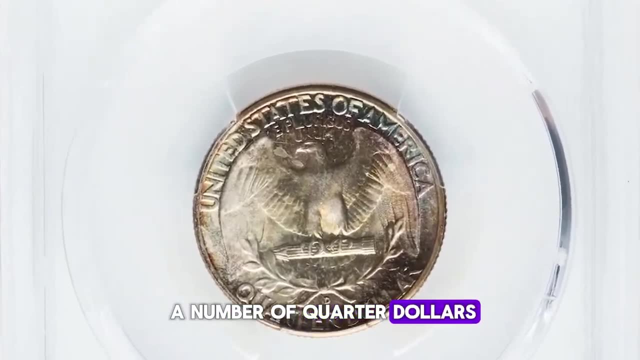 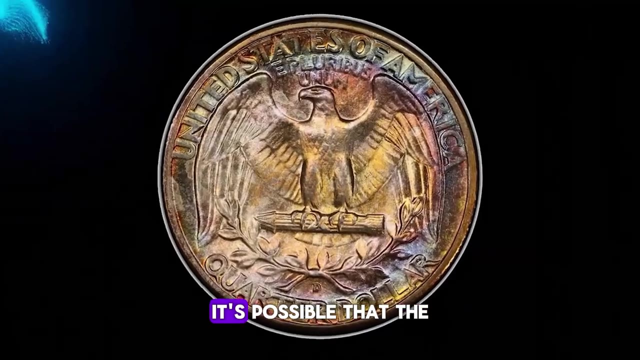 $84,000, presenting the 1942 D Washington quarter in mint state 68. Surprisingly, the Denver Mint struck a number of quarter dollars comparable to the production of 1941, despite the rapid buildup of America's economy during this time, It's possible that 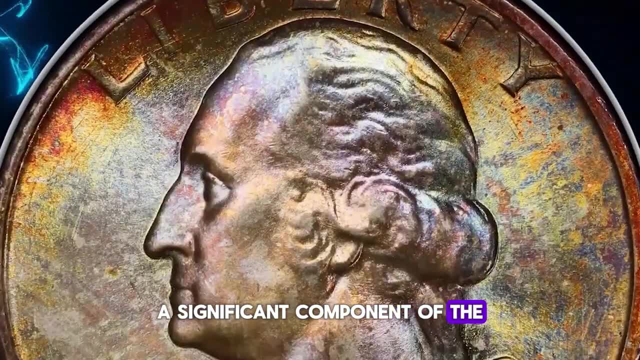 the agricultural sector, a significant component of the 1927 P cent, may have been able to make a significant contribution to the production of the mint state, but the production of the Denver Mint service territory was not as greatly affected by the production increase typical of both. 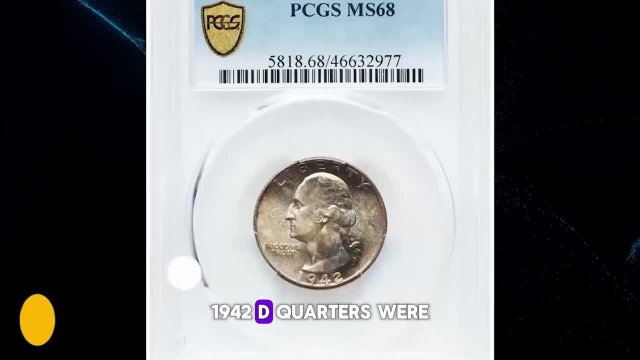 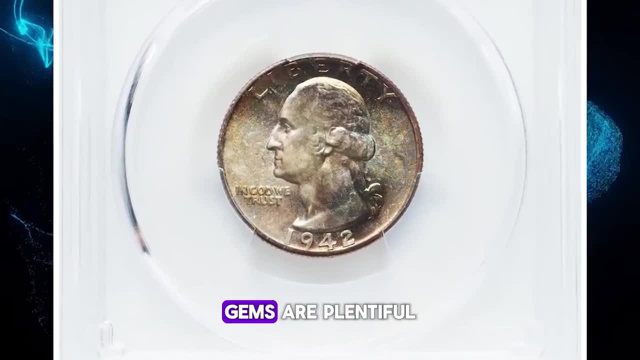 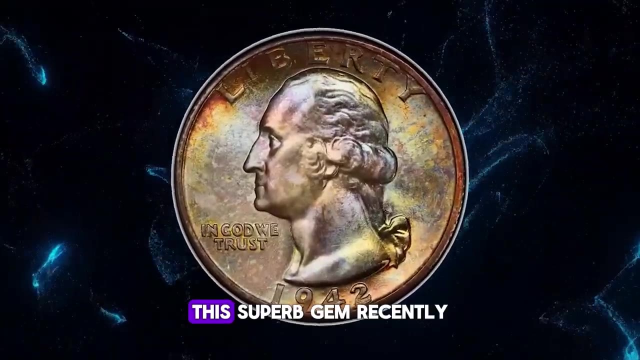 coasts 1942 D quarters were notably well-made compared to those from the other two mints, a trend often seen during the war years. Gems are plentiful, with even a fairly large number of MS67 examples available to advanced collectors. This superb gem recently sold for $4,226.40,. 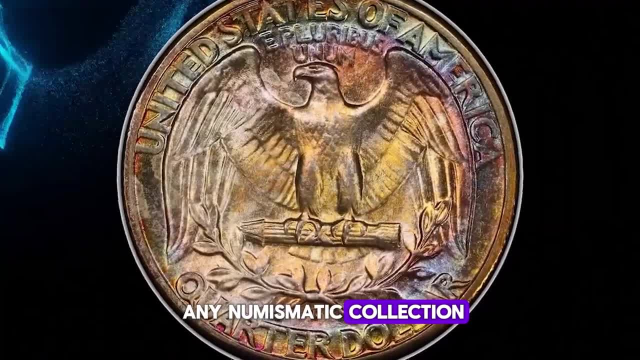 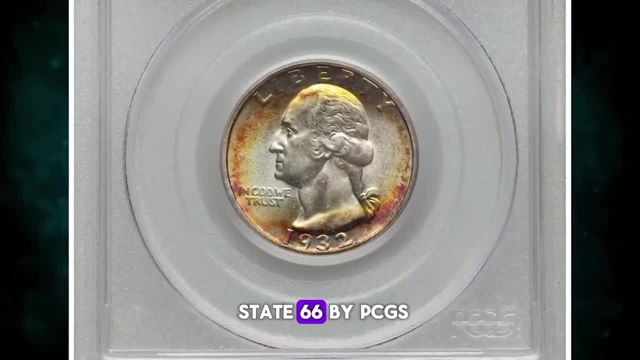 representing a pretty good price. This is a good example of a high-quality gem, a prized addition to any numismatic collection. The 1932 D Washington quarter graded mint state 66 by PCGS is one of the two key dates. 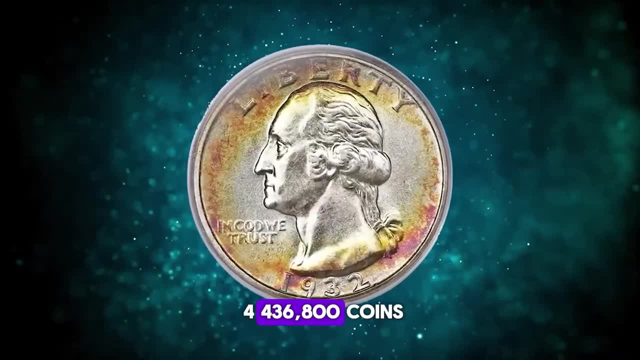 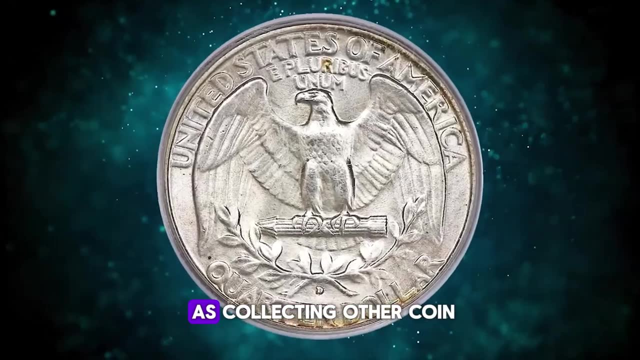 in the series. With a mintage of 436,800 coins, it has the second-lowest mintage in the series. In 1932, collecting quarters was not as popular as collecting other coin types like cents, nickels and dimes, which were inexpensive and avidly collected from circulation by the 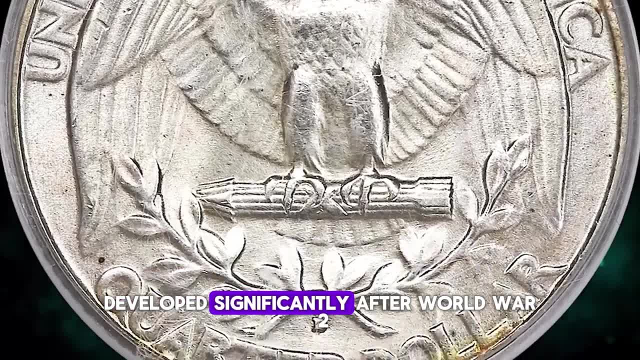 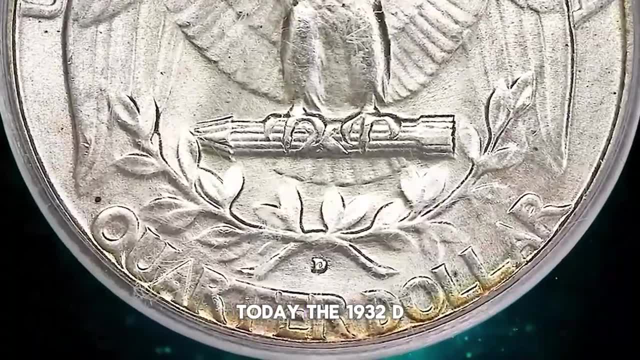 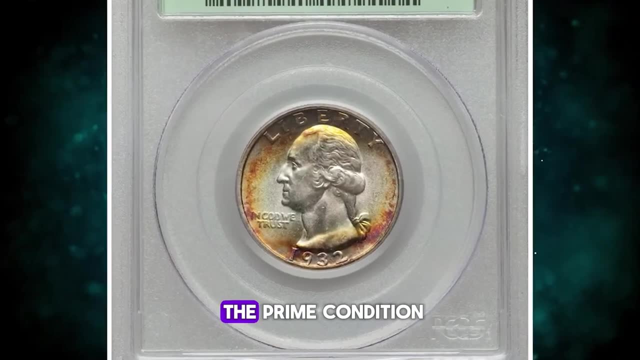 general public. Numismatic demand for quarters developed significantly after World War II and most survivors were culled from circulation by 1960. Today the 1932 D is scarce in lower mint state grades but not truly rare. However, it is considered the prime condition rarity of 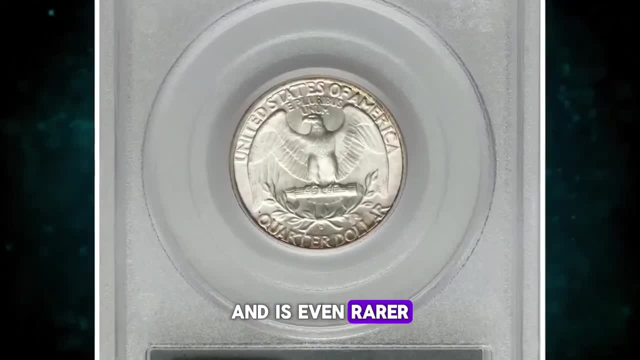 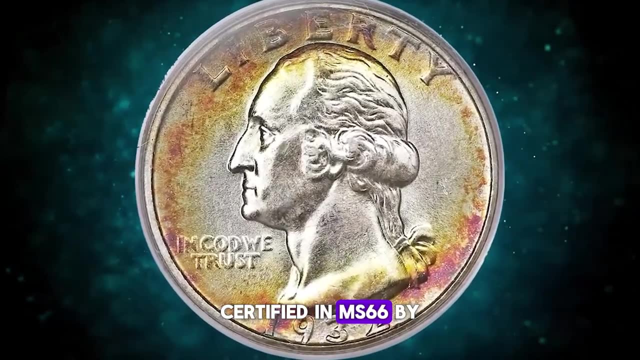 the series in gem or better condition and is even rarer than the lower mintage 1932 S at that grade level. The present coin was the first example certified in MS66, by any grading service. The surfaces are exceptionally clean and free from the abrasions.